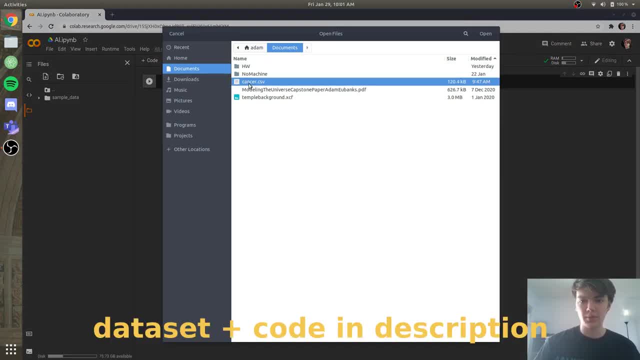 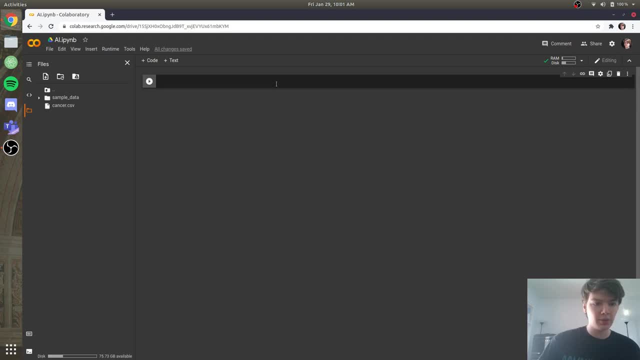 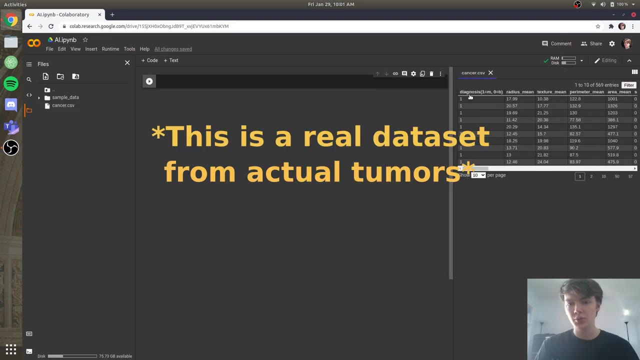 set, which you will be able to find in the description, and so the name of our data set is cancercsv. So we'll upload that and I'll show you what we're working with here. So if we double click on that cancercsv, you'll see we have a diagnosis and then we have a bunch of numerical. 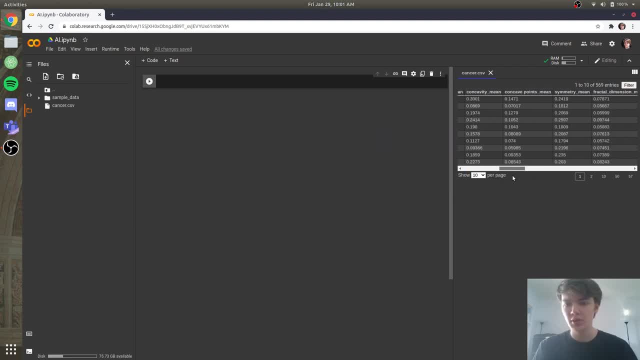 attributes relating to different tumors. Um, that may or may not be cancerous, and so what we're going to do here is we're going to make an AI figure out, based on these parameters, whether a tumor is malignant or benign. So malignant meaning that the tumor needs to be removed, and benign meaning that the tumor is not cancerous. So we 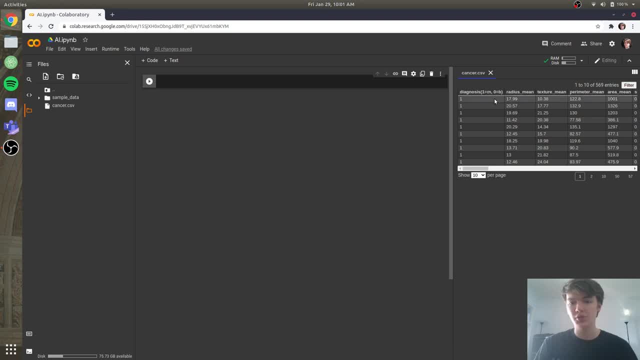 see here we have in the label diagnosis: one means that the tumor is malignant and zero means the tumor is benign. And so for radiologists, this is a very important thing to know because if you're part of their job, because they have to make sure whether or not what they're seeing on the 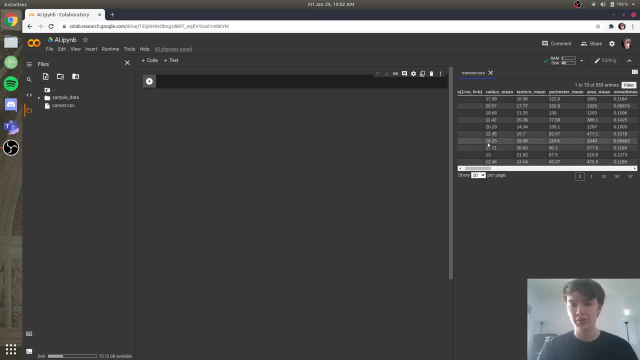 mammogram or whatever is actually going to be a malignant tumor. So having AI help radiologists in this effort is really important and can actually save lives, And we can do this in just a couple of minutes. So the first thing that we need to do is we need to import our data set And so 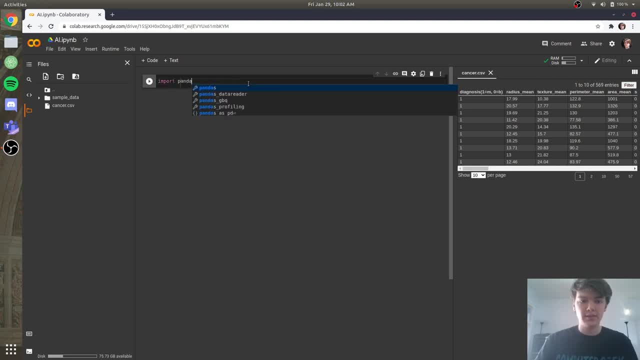 what we're going to do is we're going to import pandas as PD, and so, if you don't know what pandas is, it's a library that lets us do a bunch of cool stuff with data in Python. And then we're going to set our data set equal to pdread, underscore, csv, And the file that we are putting into our 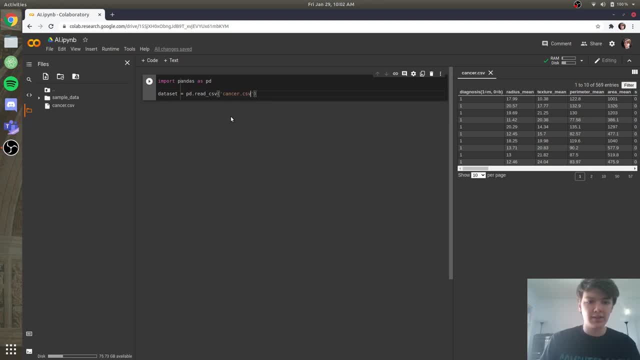 environment is called cancer dot csv. Okay, so we'll run that, And the way that you run things is unlike other files or other programs, where you run the entire file all at once. In Google Colab, you're running it cell by cell, And so, in order to run this cell, what you're going to do is: 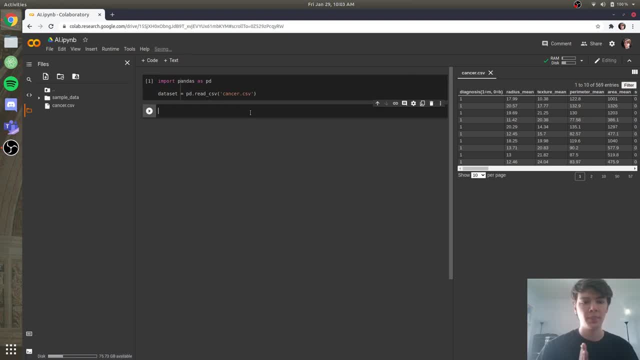 you're just going to press shift, enter and it'll create a new cell for you. So now that we know that that part of the code is working, next we need to set up our x and our y attributes. So the y attribute that we're going to be wanting to predict is whether or not the tumor is malignant or benign. 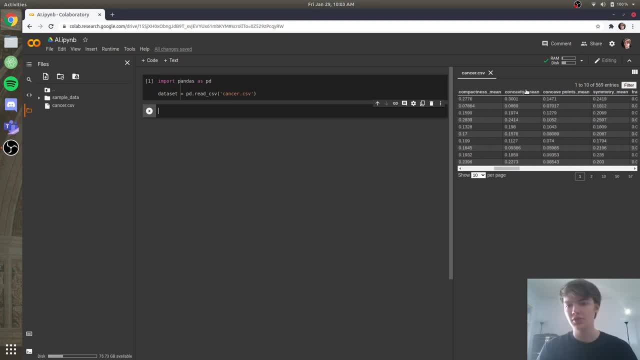 And the x attribute is going to be all of these features, And what we're going to do is we're going to have the AI map the correlations between these two features, And that will allow the AI to predict whether or not a tumor is malignant or benign. So, in order to do this, we're going to say: our x is going to equal. 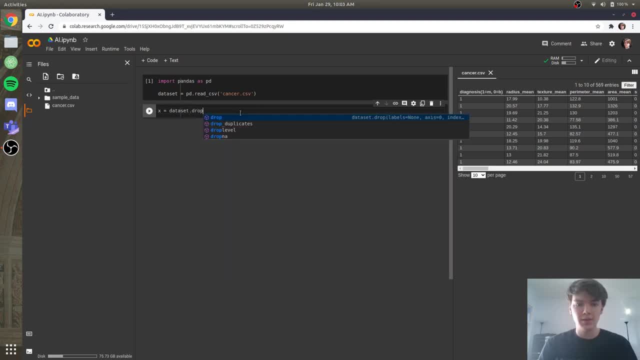 to data set dot drop, And when we're dropping, what we're basically doing is removing a column. So our data set dot drop and we are going to drop the column which is called diagnosis. one equals m, comma. zero equals b, close parentheses. And so with that, all we've done is we've 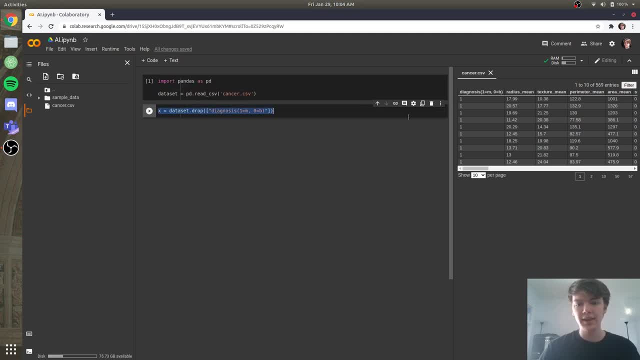 said that our x attribute is equal to everything in the data set except for this diagnosis column. So we'll run that And it says this isn't found in axis And that's because we need to say the columns that were dropped. So what we're dropping is just going to be the diagnoses. and one equals m, zero equals b. 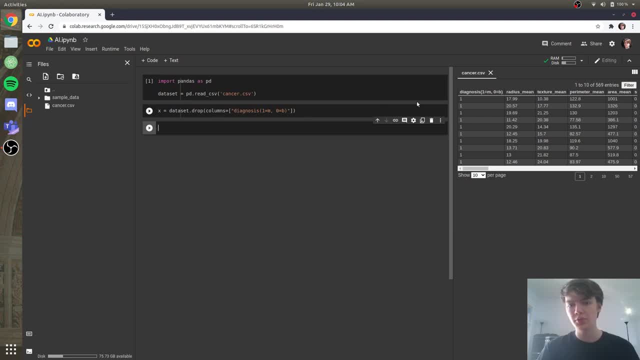 So we'll run that And then for the y column, all we're doing is we're taking the diagnoses column. So y is going to be equal to data set And the column is going to be diagnosis. one equals m, zero equals b. 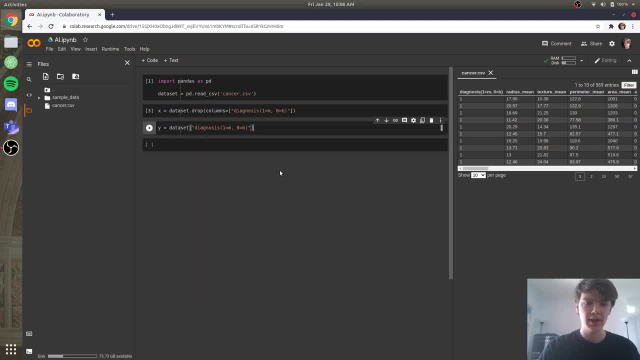 So we'll run that, Okay. so now we have our y column and we have our x column. All that's left is to split up our data between a training set and a testing set, And this is something that's really, really important in artificial intelligence, because oftentimes 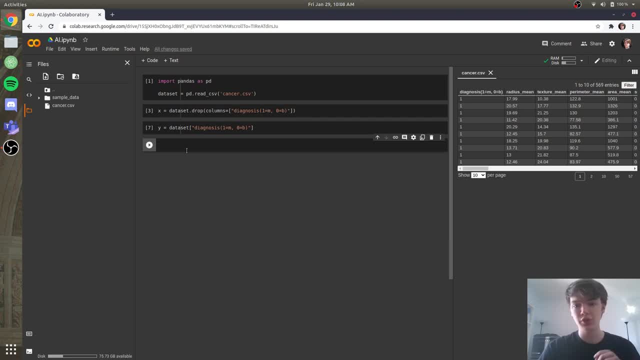 you'll find algorithms are overfitting, which means that they do really really well on the data that they've already seen. that's going into the algorithm, But when you give them new data, they just fall apart, And so, in order to mitigate this, what we're doing is we're going to set up a training set. 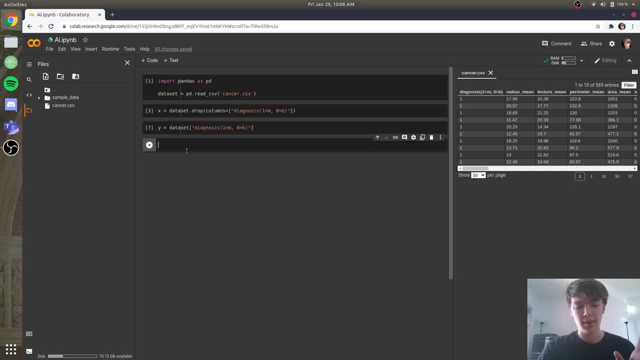 We're going to set apart part of our data, set aside to be tested on later with our algorithm. So the algorithm will be given data that's never seen before And then we'll use how well it does on that data to evaluate it, because that's really what we're looking for. 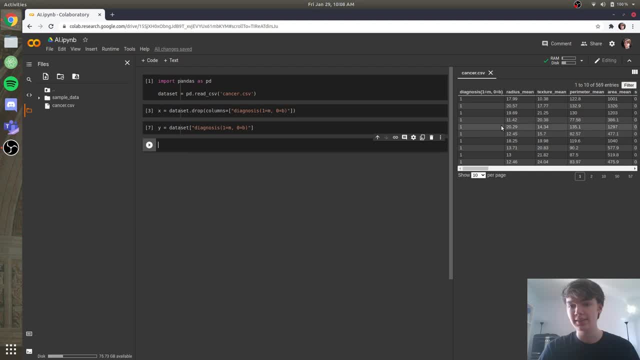 Not how well does the algorithm understand the entire data set, but more just the problem in general, which is cancer diagnoses. So what we're going to do is we're going to say from sklearncom Model selection And so scikit-learn is actually a really popular machine learning library. 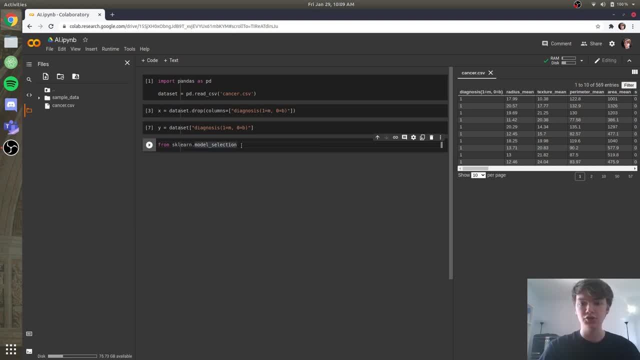 We call it sklearn when we import it, And I have an entire tutorial series on how to do it which you can check out in the card. But today we're actually going to be using another library mainly, but we're going to still use. 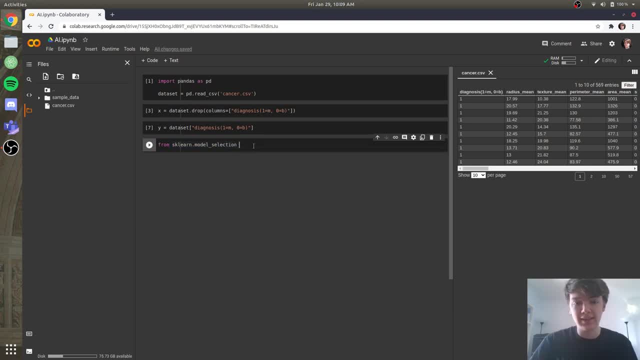 scikit-learn just to split our data set in between a training set and a testing set. So we'll say import train test splits And then we're going to say our X train, our X test, our Y train and our Y test is going to be equal to that train test split. 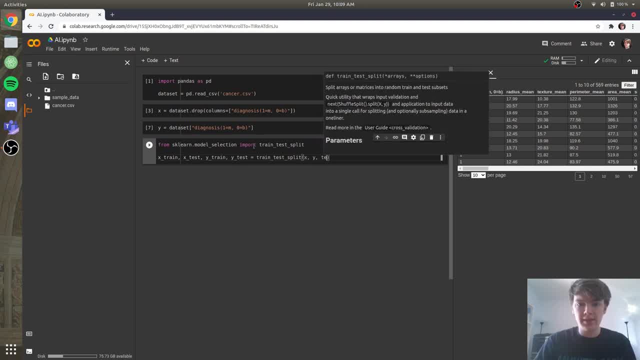 And we're going to do the split on X and Y And the test size is going to equal to 0.2.. So basically, 20% of our data is going to be in the testing set. All right, And that's actually a pretty, pretty normal way to divide things up. 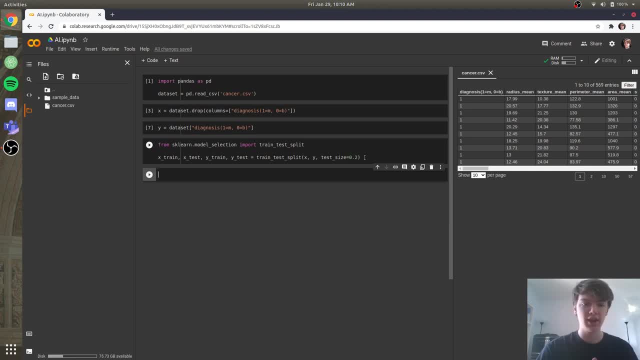 80-20.. Awesome. Now it's actually time to build our artificial intelligence, And we're going to be doing this using TensorFlow's Keras, which is really, really popular, And we're actually going to be building a neural network, which is also a very, very popular form of AI that can be used in almost any problem. 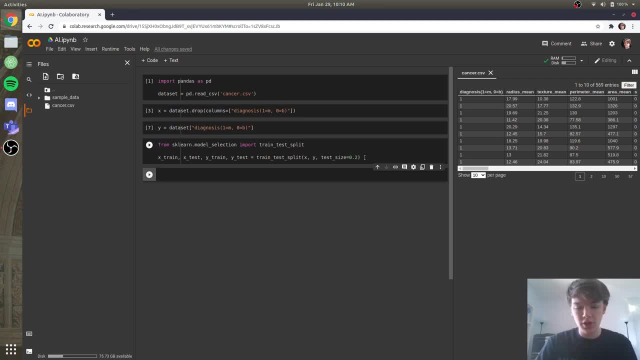 And it just sort of adapts to it. So, in order to do that, First we're going to import TensorFlow As TF And we're going to say: our model is equal to TF, dot, Keras, dot, models, dot, sequential. Okay, so we have that. 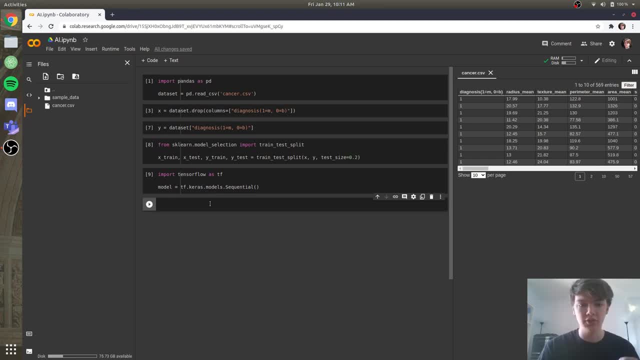 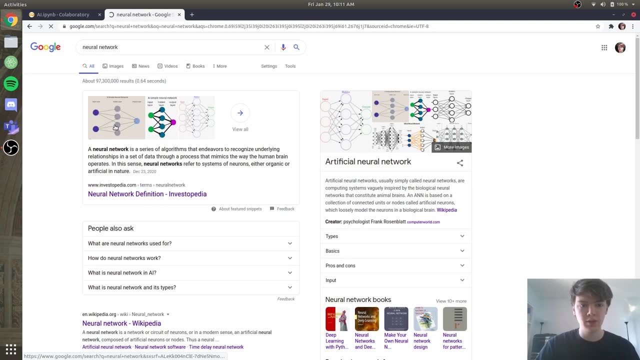 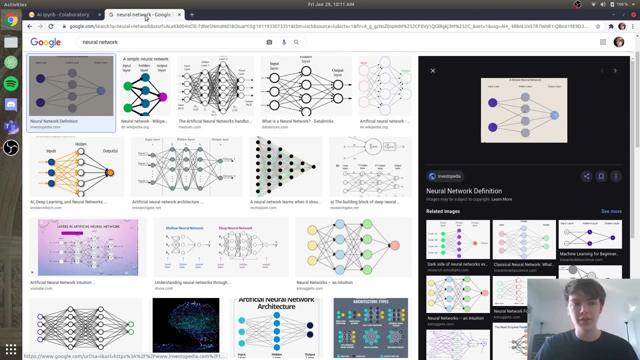 And everything looks good there. Next, we need to start adding layers to our module. So if you look up a neural network, what we have here is we have an input layer which is our x values, all the different attributes of the cancer data set. 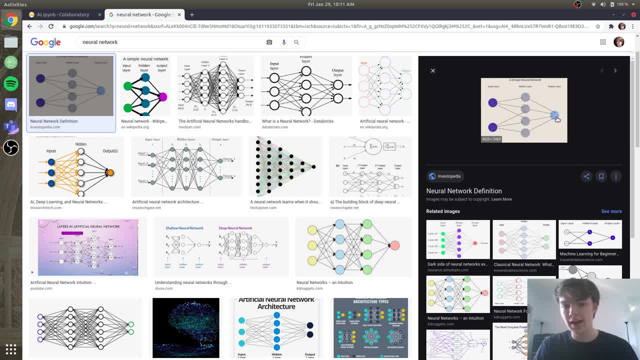 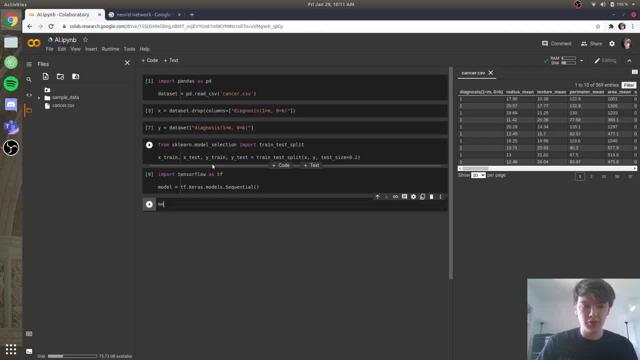 And then it goes through a hidden layer And then finally there's an output layer which would tell us if our tumor is malignant or benign. Okay, so we're going to do is we're going to say model, dot add, And we're going to add TF, dot. Keras, dot layers, dot dense. 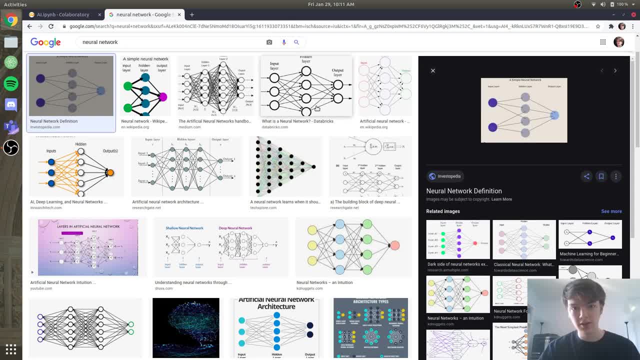 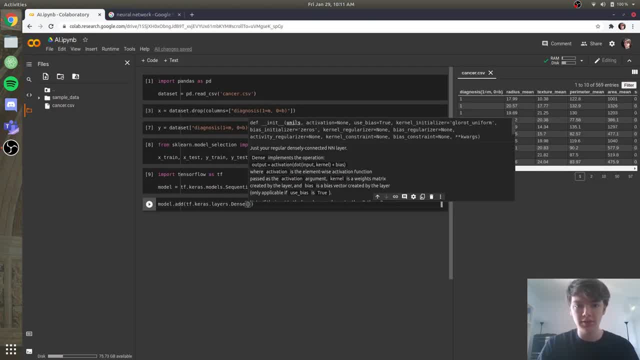 And so what a dense is is a dense is just one of these standard vanilla sort of default neurons that you get in Keras. And so the number of units we want- and you can see here it says: input the units- We're just going to give it some random power of two. 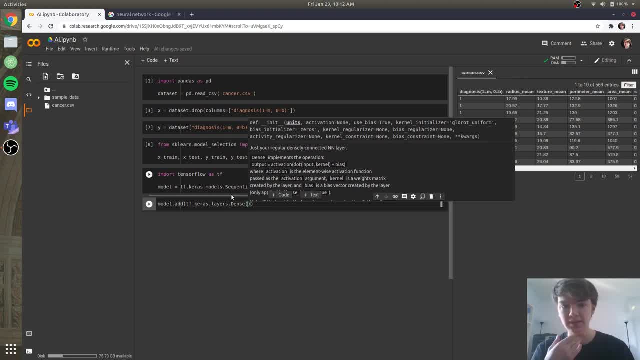 So I'm going to make this neural network really, really big, bigger than it needs to be, just to sort of see How powerful we can get with this data set. So we'll say 256.. And then, since this is actually our input layer, we need to say that the 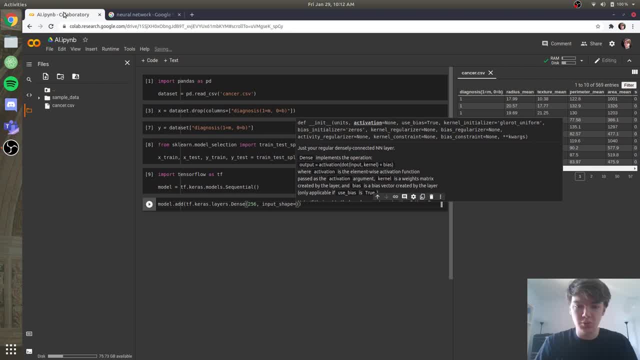 input shape is equal to, and it'll be equal to, the x train dot shape. Okay, So basically what we're saying is we're going to input something with the size of the x train dot shape, which is to say, all of these x features right here. 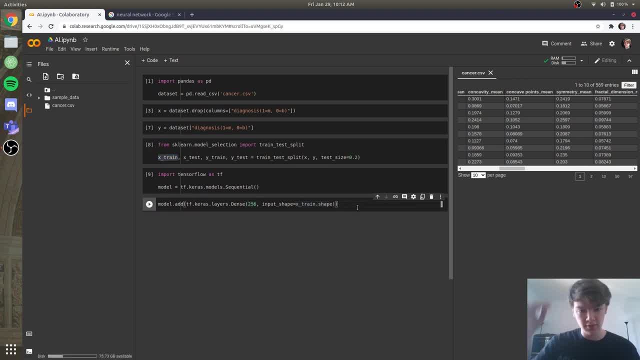 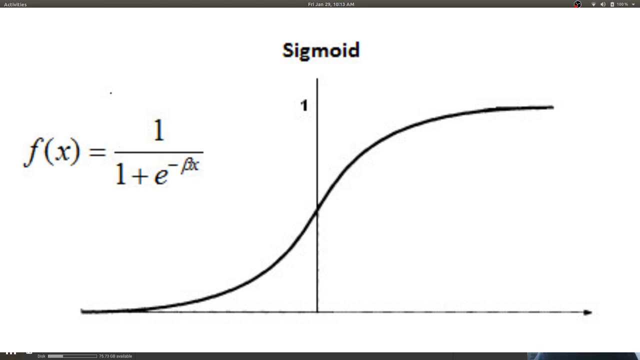 And then the output will be 256 neurons. And then, most importantly, we also need an activation function, Which we're going to set to sigmoid, and basically all the sigmoid function is, if you see on your screen Now we're taking all the values from the neural network and we're just plotting them between 0 and 1, and this is going to be very 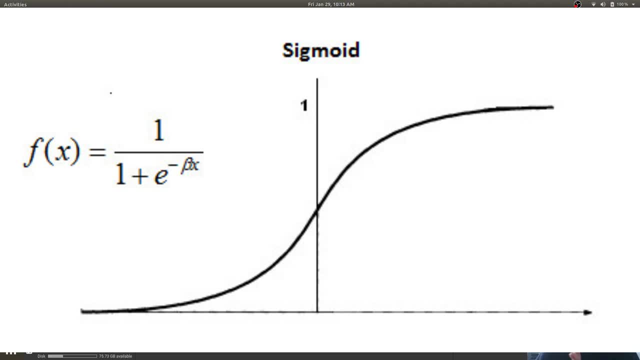 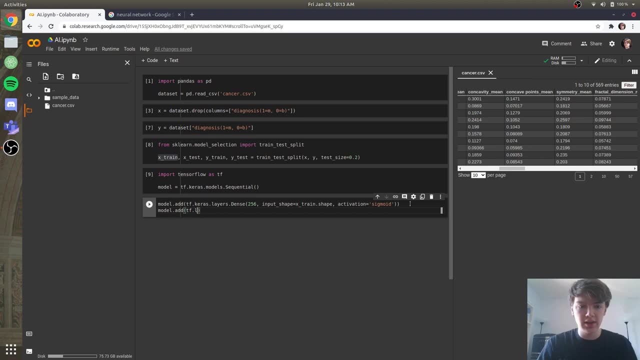 helpful for reducing model complexity and also making the model more accurate. So now let's add another layer, We'll say model dot, add tf, dot, keras, dot, layers, dot, dense. And let's say let's get another 256 neurons And also the activation function will be sigmoid. 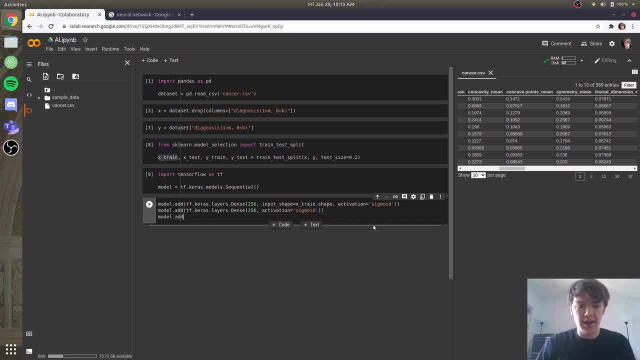 And then finally, let's make our output layer. We'll say model dot, add tf, dot, keras, dot, layers, dot, dense, And we'll just have one dense neuron with the activation function sigmoid, Because again, our final value is just going to be one single value between 0 and 1 for the diagnosis. 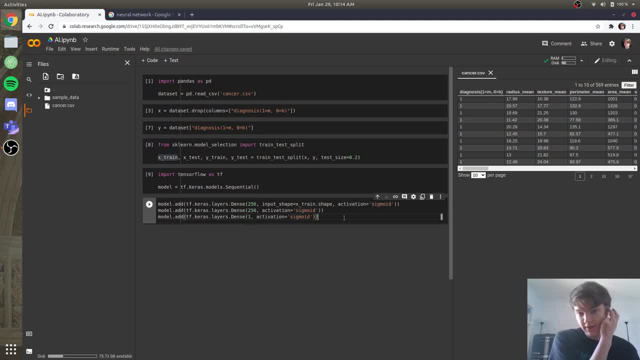 So you can understand why sigmoid function works. Sigmoid function might be helpful in that scenario. Okay, so we'll run this And it looks like everything ran. Okay, So next it's time to compile our model. So we're going to say model dot compile. 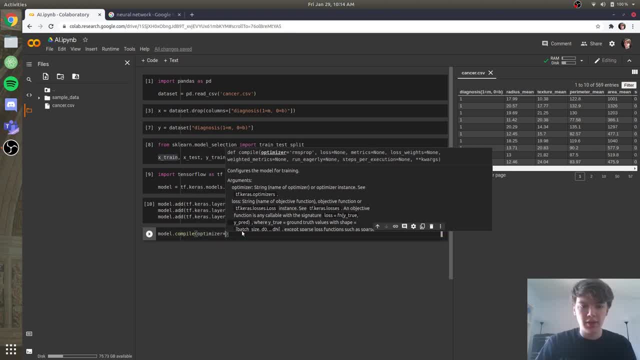 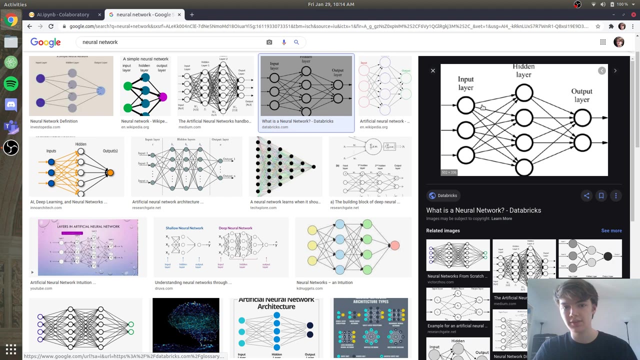 And what we need is we need an optimizer. So the optimizer that we're going to be using is called Adam, And you can see more information about how this works, But this is basically how the machine learning algorithm is being optimized, how the neurons, how the weights of the algorithm are being fine-tuned to fit the data. 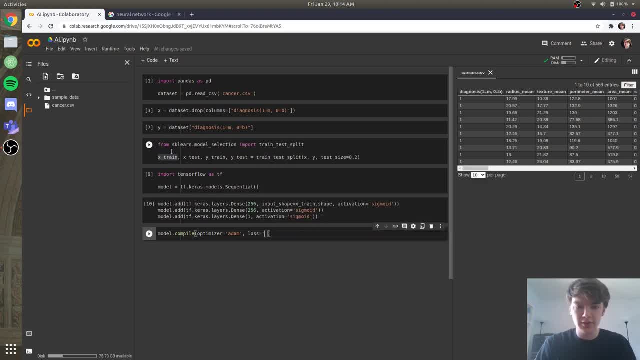 Next, we're going to have a loss function, And so the loss function because we're doing binary classification, we use an algorithm or we use a metric called binary cross entropy, And this is really really good when we're talking about categorical stuff. 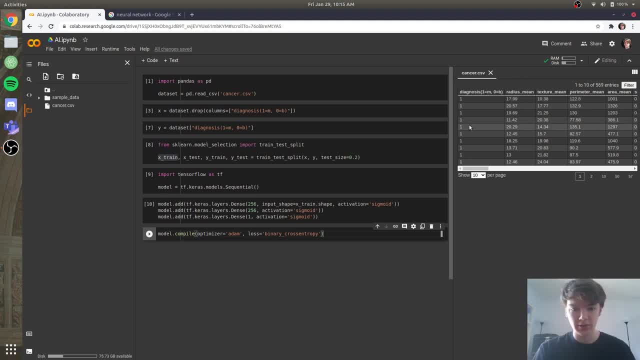 So like malignant or benign, just discrete values like that, And then, finally, the metrics that we're going to be looking at is we want to look at accuracy, because we want to correctly classify as many tumors as possible, So we'll run that. 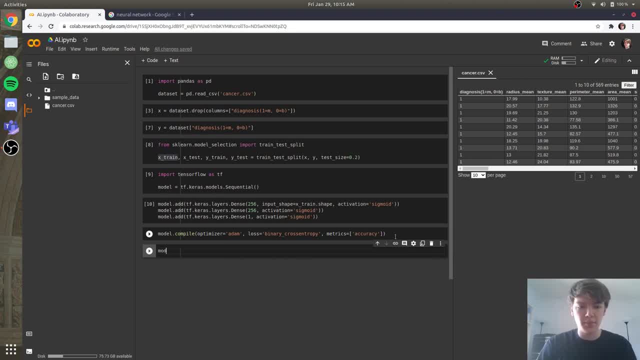 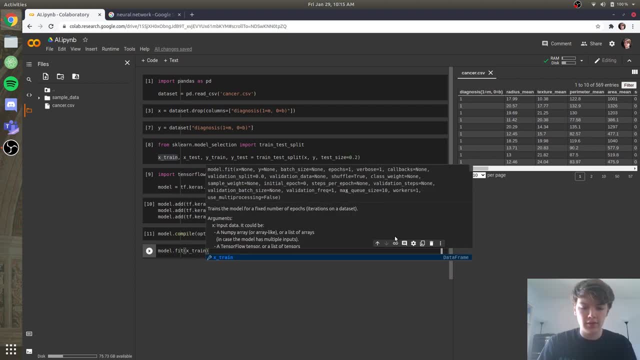 Awesome. Now it's time to fit our data. So we'll say model dot, fit, and we're going to fit the X train of our model To the Y train And we're going to set the number of epics to, let's just say, a thousand. 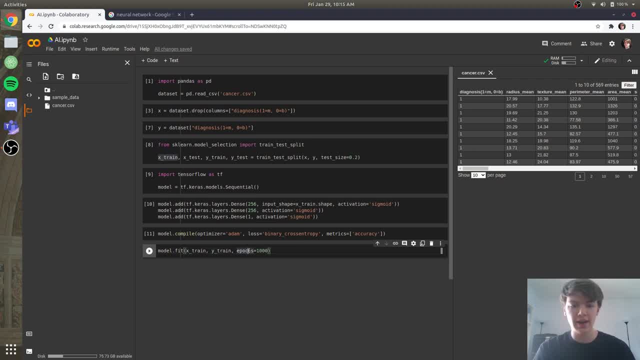 And so what the epics mean is that that's how many times our algorithm is iterating over the same data. So usually on the first run through the entire data. especially with a smaller data set like this, only about under 600 entries- the algorithm needs to constantly learn by going over the same data over and over again. 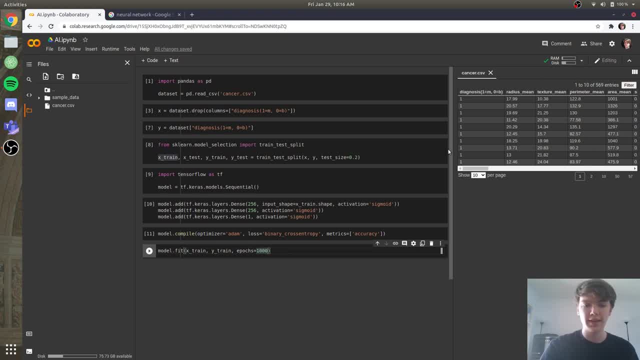 So a thousand epics is kind of a lot, but since our data set is small, that's okay, Most likely because of the size of our neural network. for the size of the problem This is a bit overkill, but it's better to be safe than sorry. 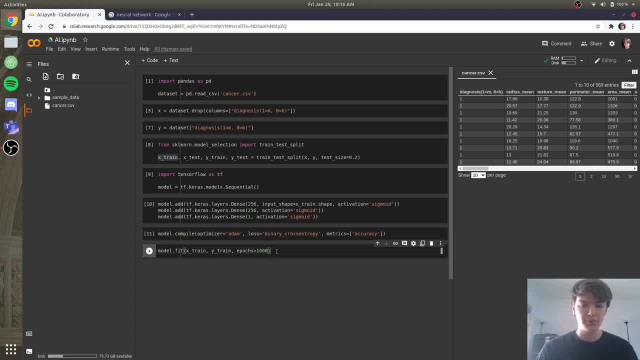 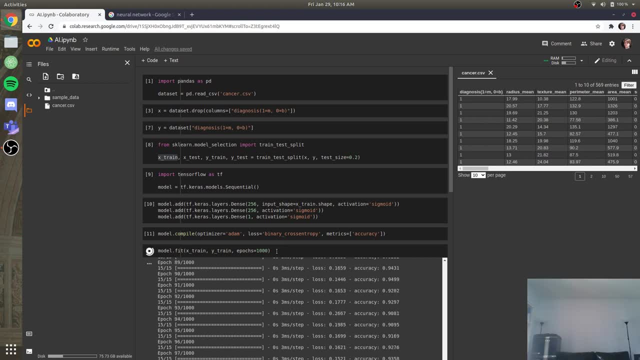 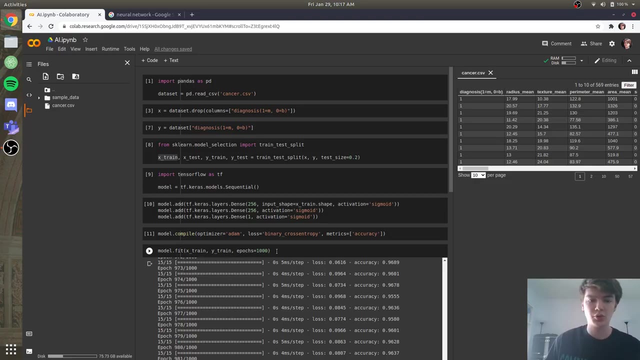 So we're going to run that and then, while that's running, I'm going to go do some push-ups A few moments later, All right? So now that I got some quick reps of push-ups in, let's see how well our model did. 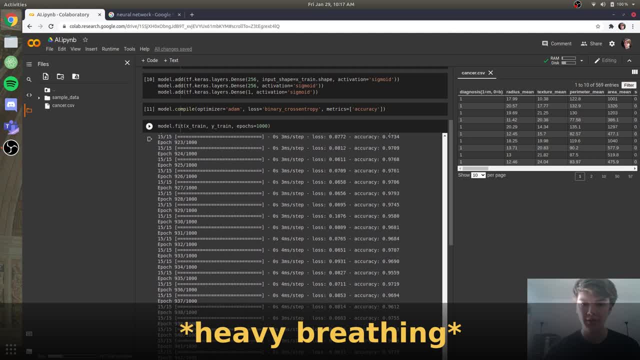 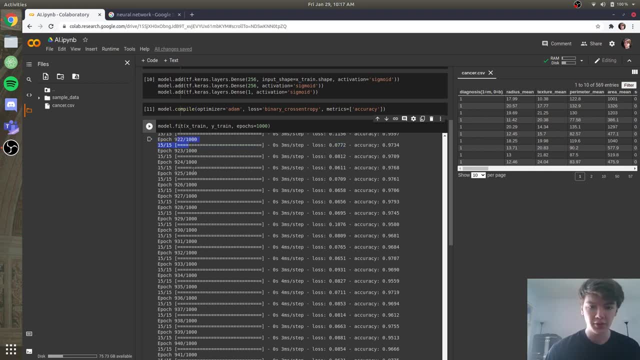 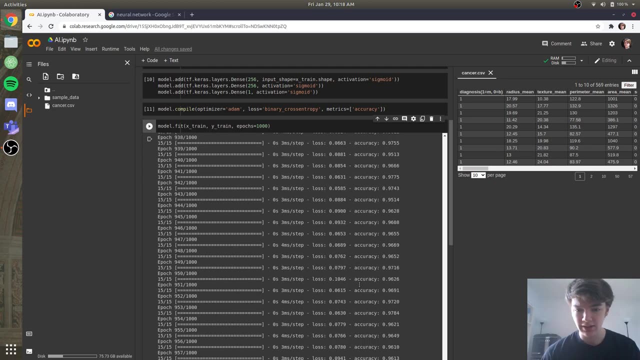 So if I scroll down you can see we have the loss function, the accuracy and also the epic that it's on. So as we're nearing towards the end, it looks like the accuracy fluctuates quite a bit, but it stays consistently above 95%. 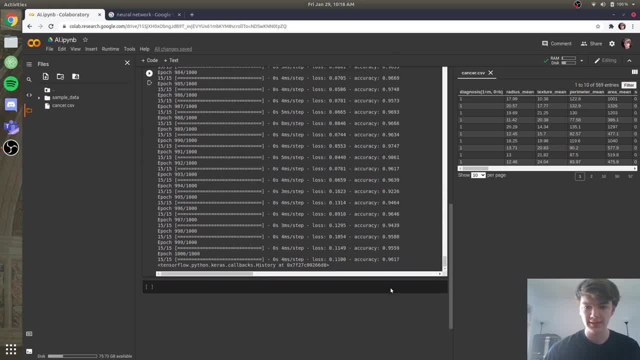 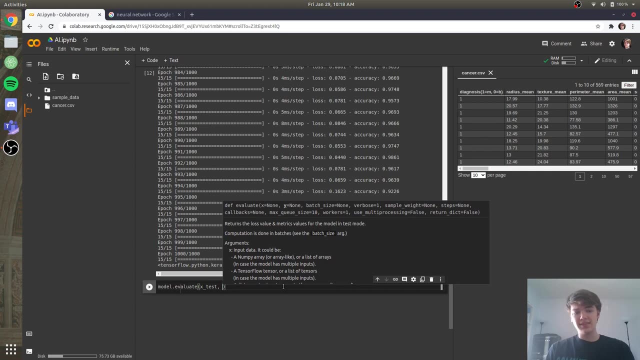 for the testing set or the training set. And now the final thing we need to do in evaluating our algorithm is we're going to say modelevaluate and we're going to evaluate with the X test. That's our testing set on the Y test. 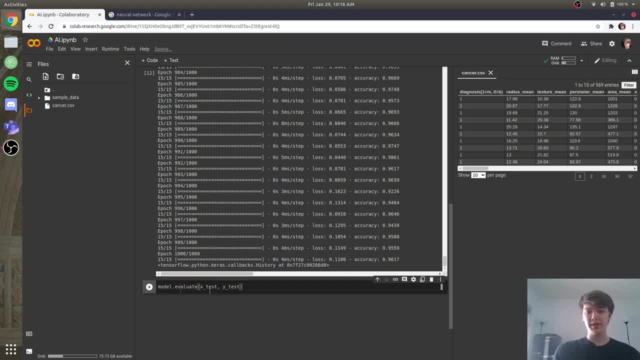 So basically, what this is doing is it's comparing what the model thinks that Y test should be versus what Y test actually is. So we'll run that And you see, our accuracy is 97%, which means that, on new data, our machine learning algorithm. 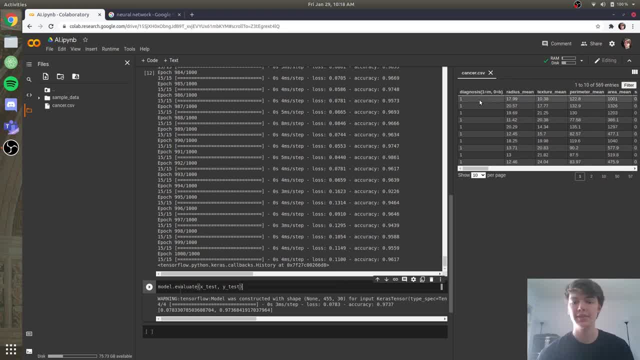 our AI can correctly classify cancer, diagnoses cancer tumors, with 97% accuracy, which is amazing considering the fact that this algorithm never went to college, didn't go to medical school, doesn't even know what a tumor is. But from this data, 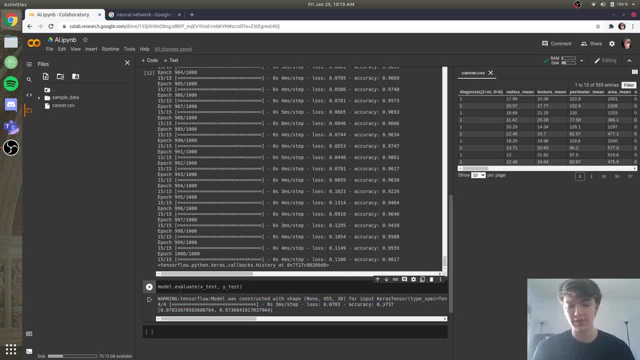 it was able to find a pattern and from that it can be used to help radiologists and doctors. So yeah, guys, that's pretty much it for this video. If you have any questions, let me know and I'll see you in the next one. 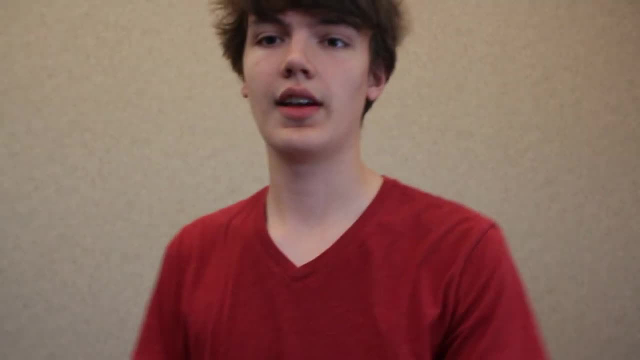 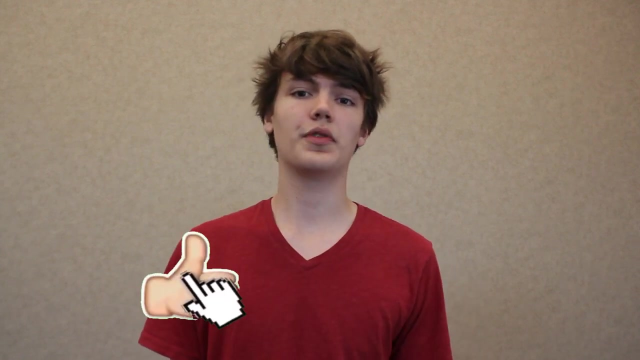 Sweet. Thank you, guys, so much for making it to the end of this video, As always. if you enjoyed it, make sure to hit that like button Also, if you have any questions, comments or concerns about what we did in this video.